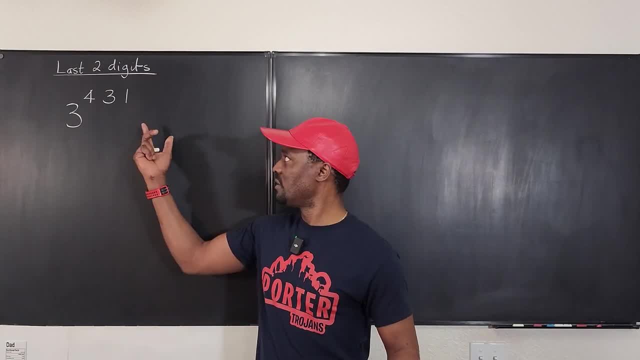 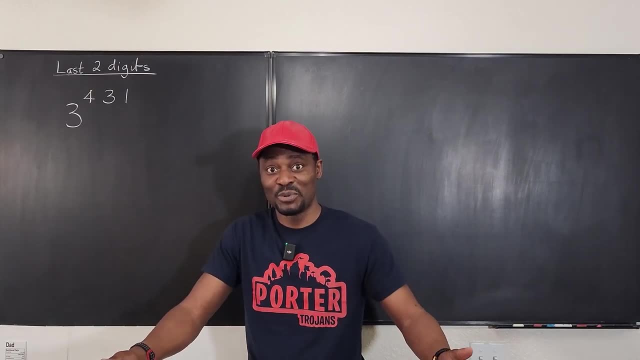 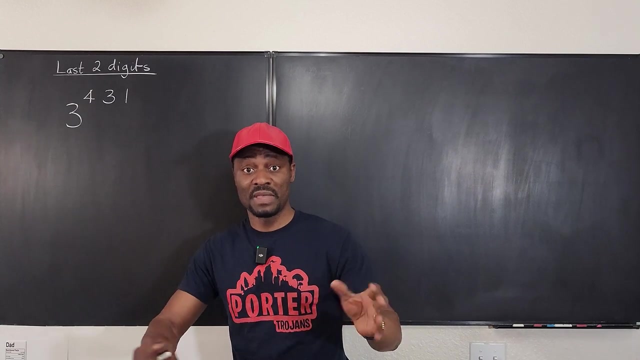 someone says: what are the last two digits of this number raised to Boy? that's a huge number. Even your calculator cannot give you the answer because you can't see the whole numbers. You have to write it in standard form with exponential function. But if you had a computer or a program that can, 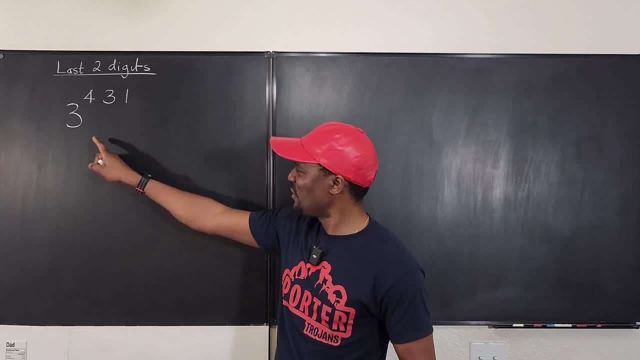 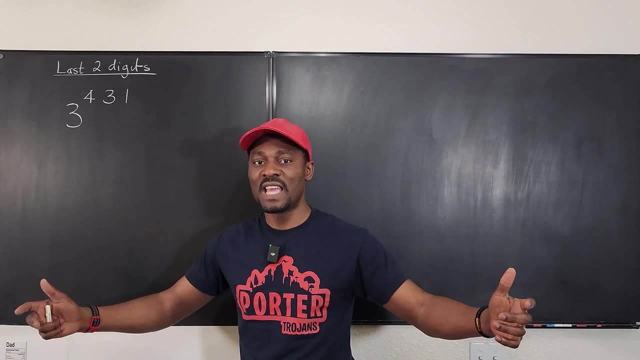 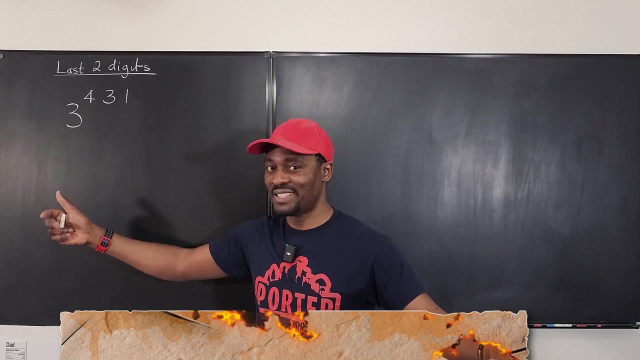 give you all the digits, you'll end up seeing what the last digit of this is. But there's so many numbers, you write so many digits, So is there a possibility of you, without you memorizing anything, being able to find the last two digits of a giant number? Okay, yes, And that's what I'm. 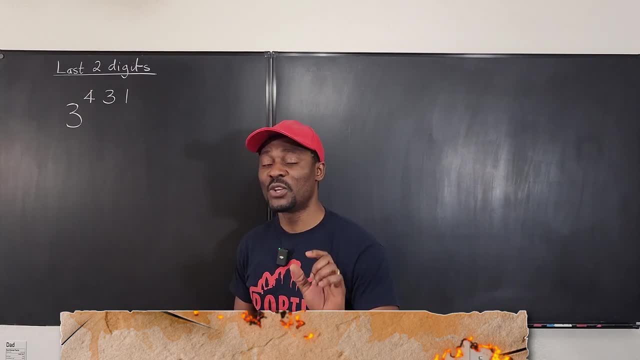 about to tell you. So look, you've seen problems like this before, where someone says: what are the last two digits of a giant number? Okay, yes, And that's what I'm about to show you in this video. Now we're going to use something called Euler's theorem and we're going to use another thing called 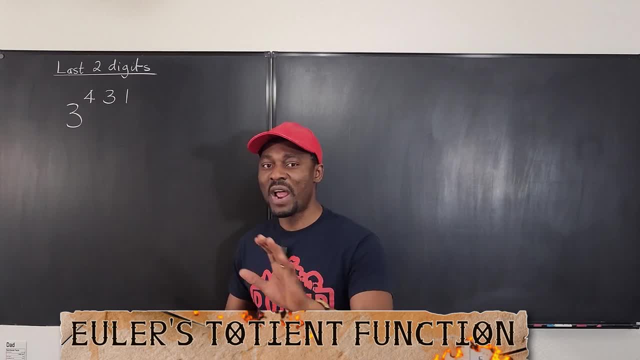 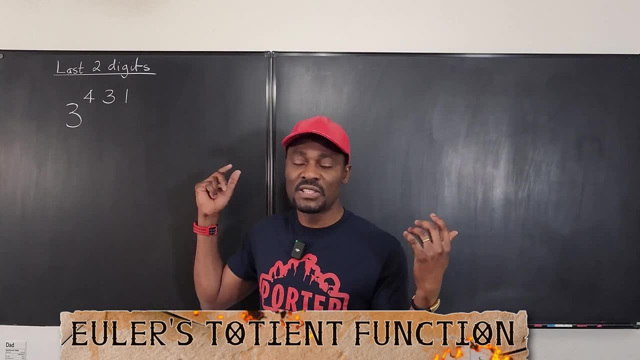 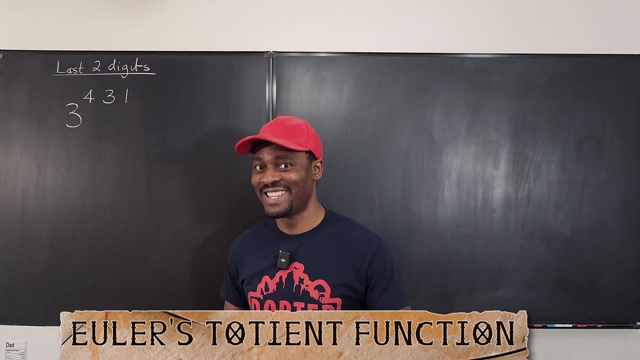 Euler's quotient function. So let me write the formula you're going to use and what it means and how you can use it for any other number, including even if it's not the last two digits. What about if it's the last digit? What about if it's the last three digits? Okay, you can do it The same. 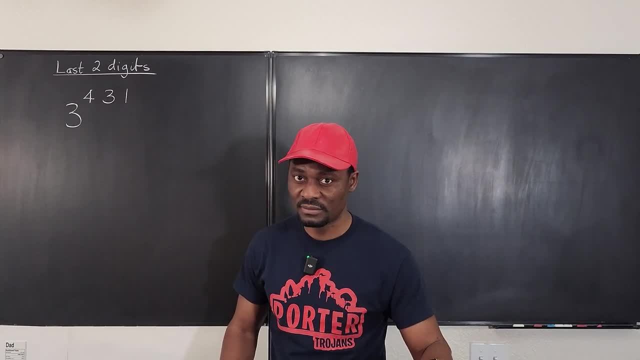 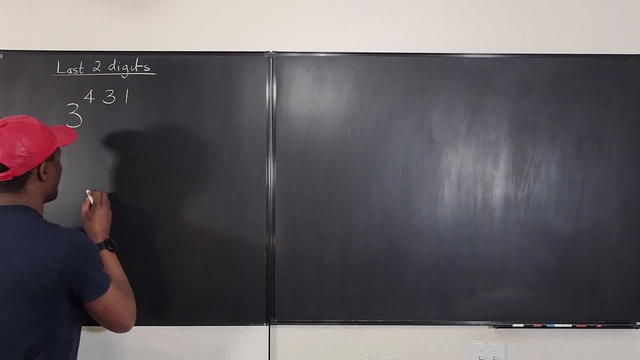 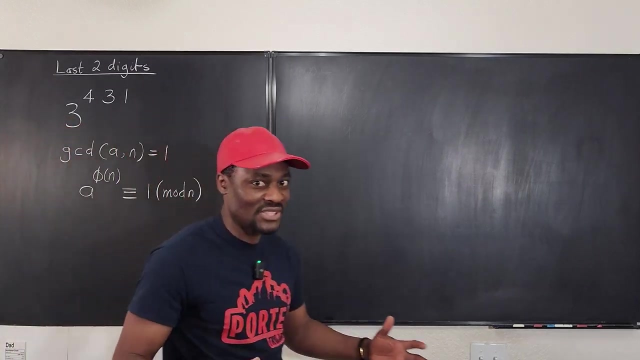 rule applies. Okay, firstly, what's the formula? The formula says: if you have any two numbers, okay, let's write that. So, if you have any two numbers, such that the GCD of those two numbers is one- I'm going to explain what this means- Then, if you raise one to the phi of n of the other, your answer will always leave a remainder of one every time you divide it by n. Okay, now this sounds like magic, but it's not. 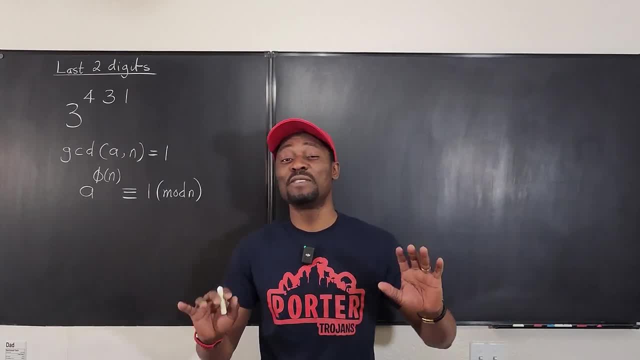 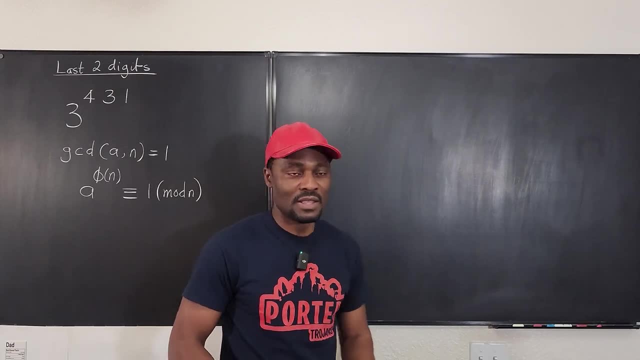 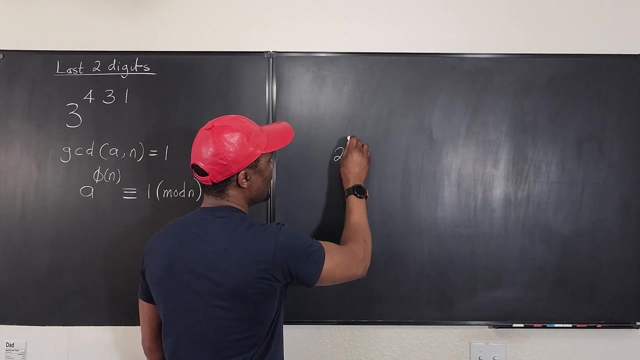 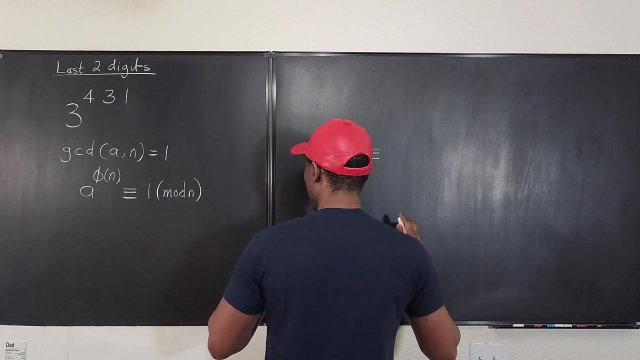 Because everything has a meaning. Let me explain to you. I'm going to use a very simple example. Let's use the two numbers, two and five. they're small, Okay, so let's say I write two, raised to power, the phi of five. My claim based on this: firstly, let's go here, see if the two of them satisfy this condition. What does this mean? It means 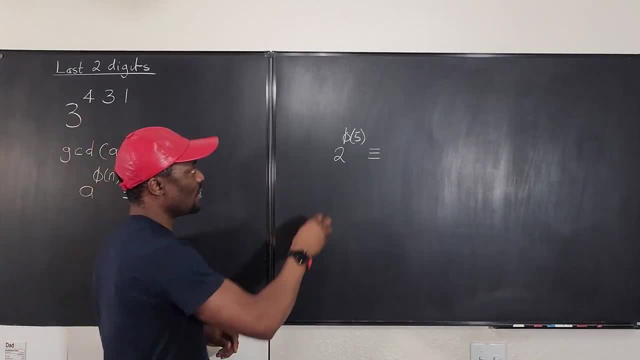 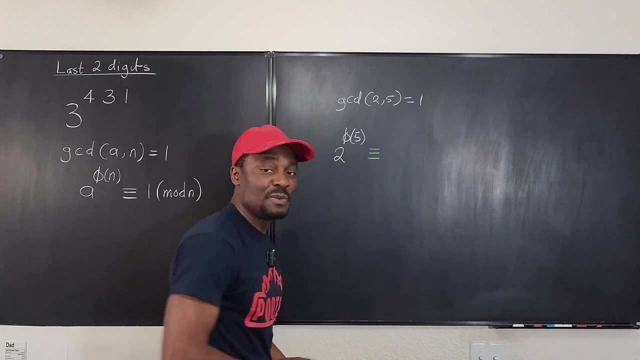 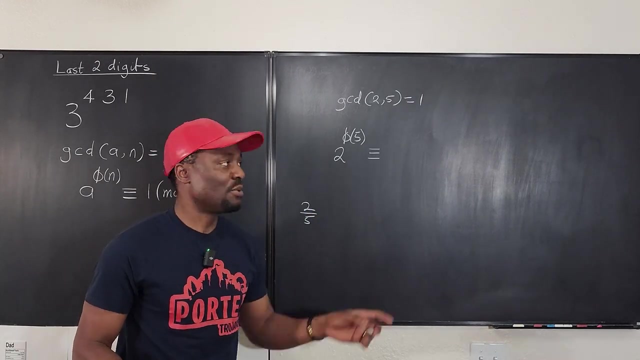 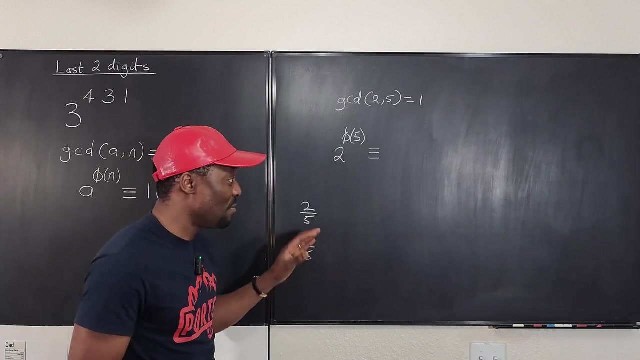 no number can divide two and five. So we say the GCD of five and two, which means they're relatively prime. You can write this as a fraction- two over five- and nobody's going to complain, Okay. but you cannot write two over six as a fraction. You have to reduce this. So it means if you put the two of them together as a fraction, there's no need to reduce anything. That's the meaning of relative. 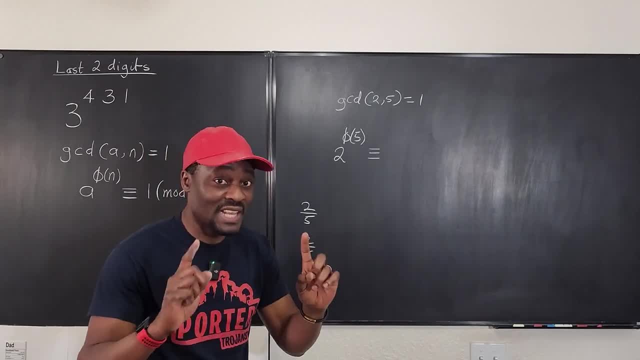 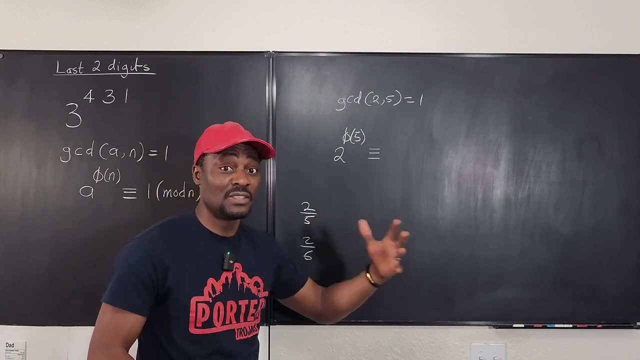 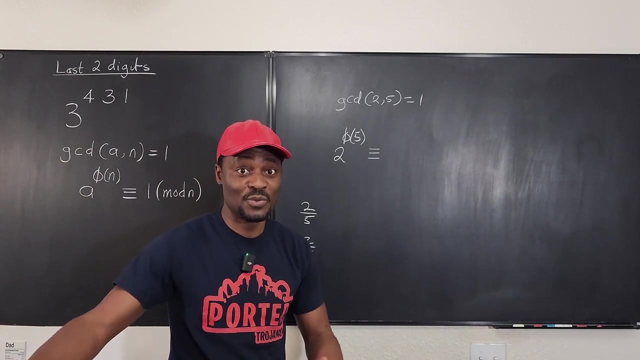 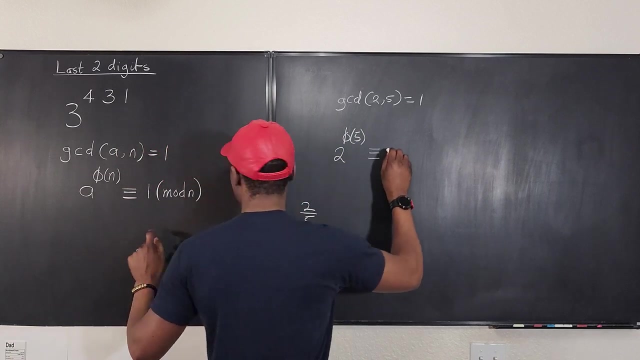 prime or GCD is one, which means the only number that can divide the two numbers is one. So you can combine two and nine, five and seven, five and 13.. You can combine 20 and three, Okay, 17 and 100,, three and 100, which is what we're about to use now, Okay, Now, basically, that's the rule. So what does this law say? It says that you're going to have one mod five. 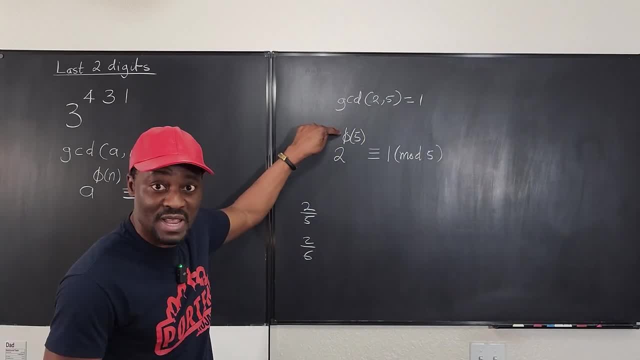 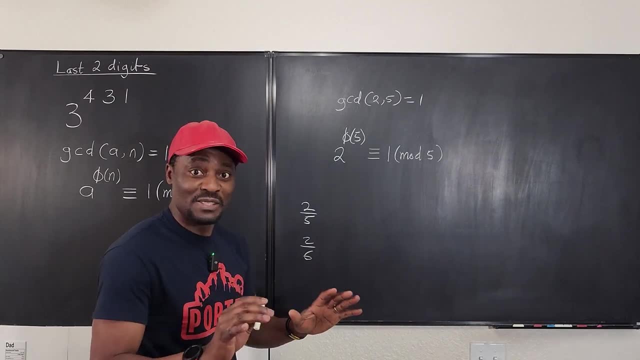 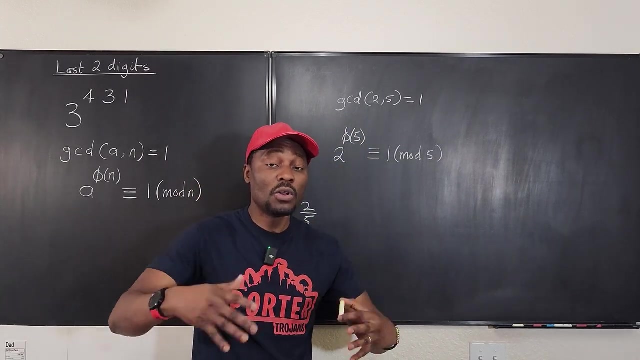 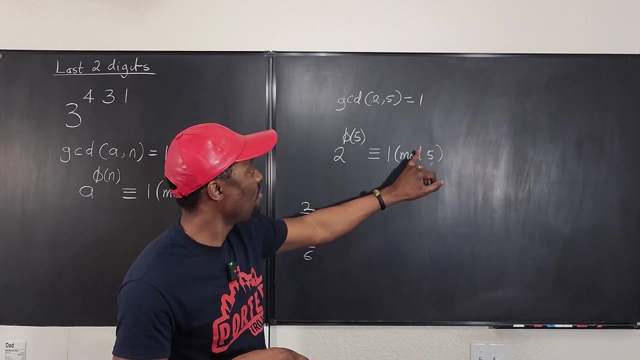 Now, what is the meaning of this? And what is the meaning of this? I'm going to explain this, okay, Because it's the first time I need to explain it, right, Okay, So what this means is you calculate the phi of five. The phi of five is the set of all numbers that do not, that are relative, that will behave like this with five, all numbers smaller than five that will behave like this along with five. So let's say you write five, What are the numbers that are less than five? 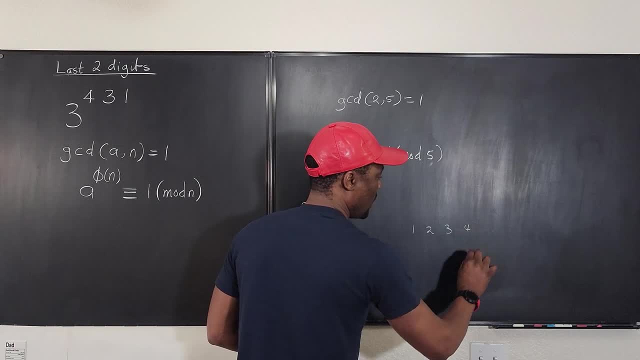 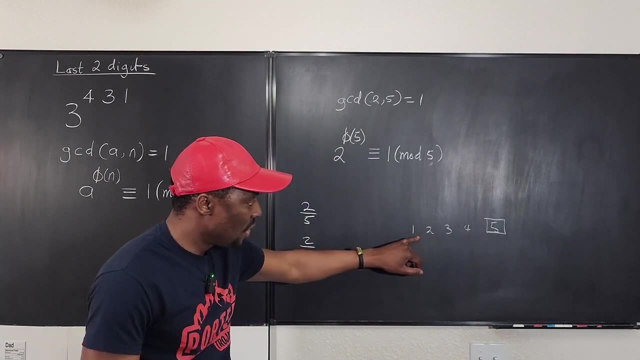 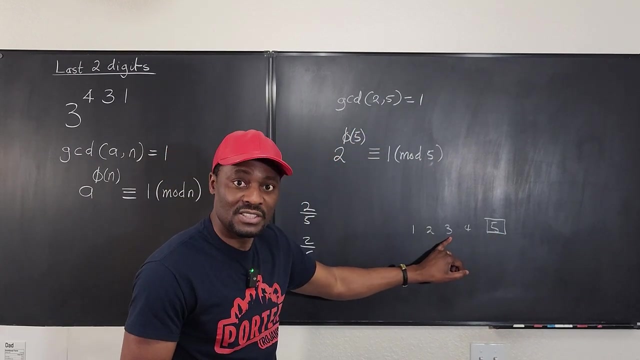 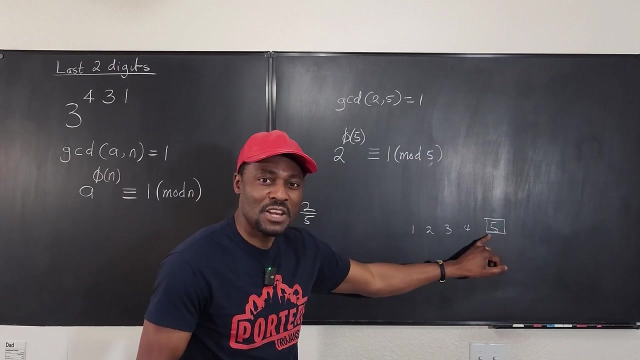 You have one, two, three, four. These numbers are all less than five. We're going to five. but one account. Now, all of these numbers, you notice that you can write them as a proper fraction because the GCD of four and five is one. That is the greatest common factor, The greatest number that can divide three and five is one. The same thing, the same thing. So how many numbers do we have? We've got four And this number. it means that the phi of five is one. 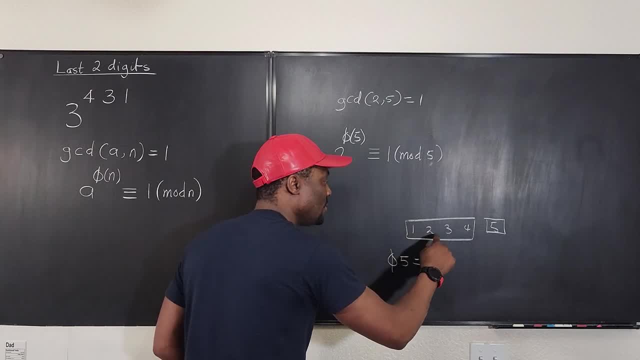 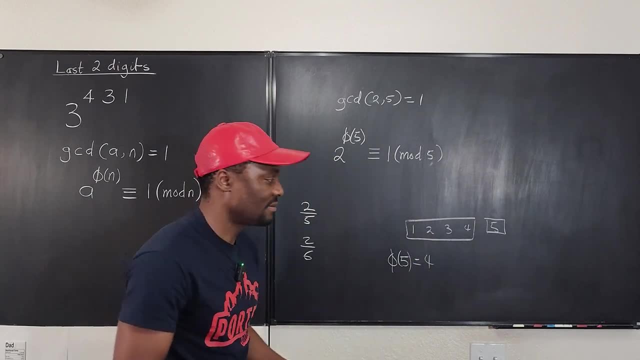 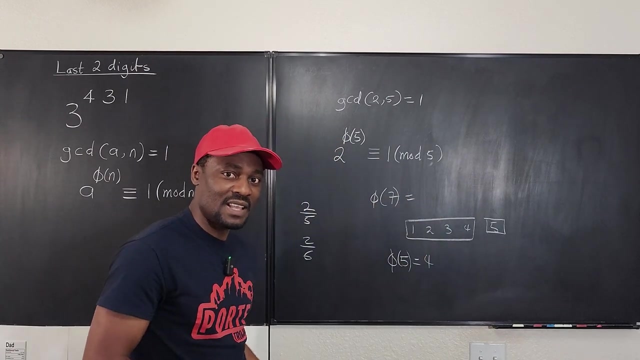 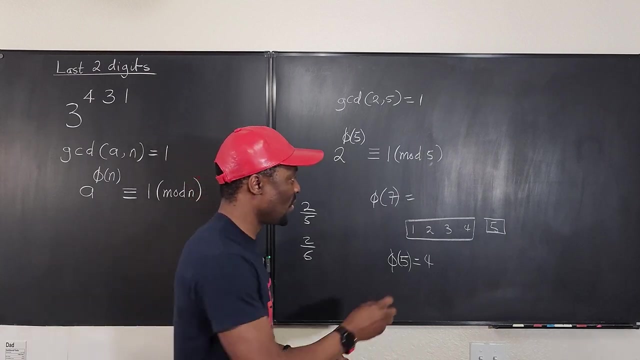 The phi of five is one plus one, two, three, four. There are four numbers that are in this category. Okay, Let's try seven. Okay, What is the phi of seven? How many numbers less than seven are relatively prime to seven? One, two, three, Oh, the numbers before seven. So the phi of seven is six. What about the phi of eight? 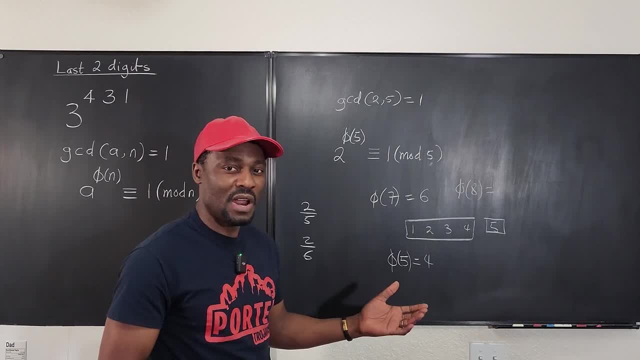 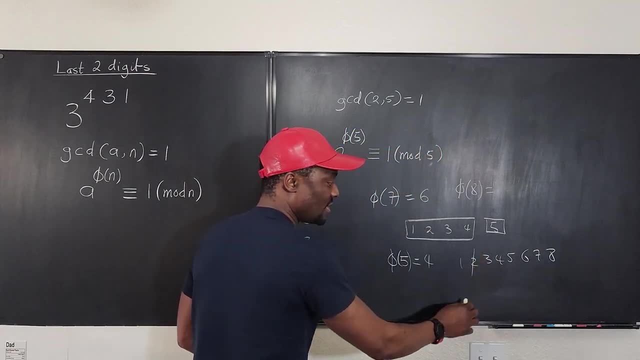 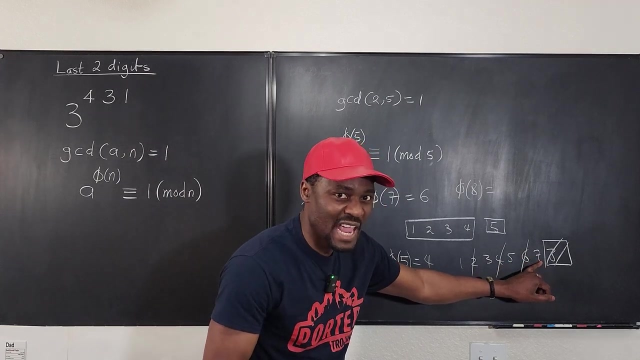 How many numbers less than eight are relatively prime to eight. Let's quickly list them: One, two, three, four, five, six, seven, eight. Well, we know that this is not relatively prime to eight, because you can't write two over eight as a fraction. You have to simplify. You can't write this and you can't write this. Sorry, This is not one of them. Okay, So one, two, three, four, five, six, seven- numbers less than eight, But out of them we've struck out three. So only one. two, three, four. Only four of them. 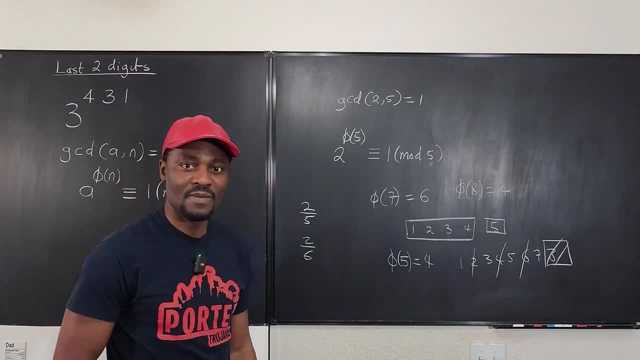 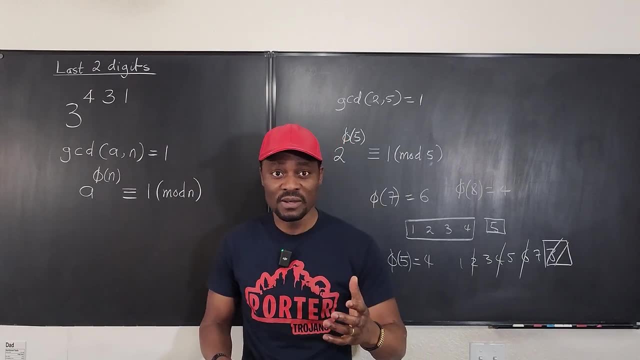 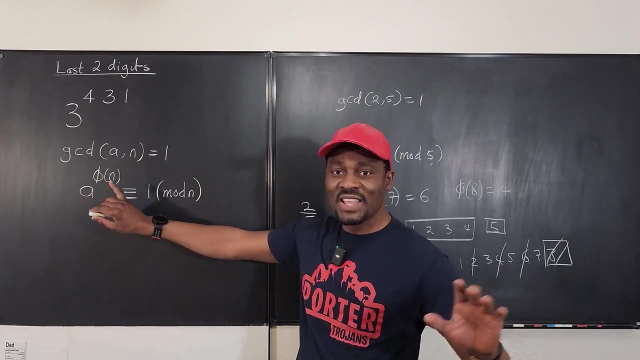 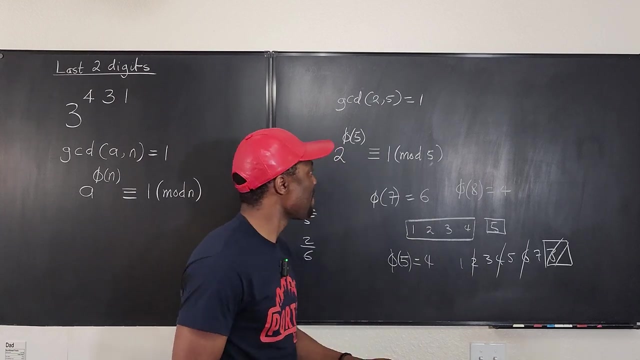 So the phi of eight is four. Now you understand what the symbol means. It's crazy how people think. But this guy called Euler invented this function called Euler's Tautient function. So this is Euler's Tautient function, And it's beautiful, So useful. Now, why do we need to use this? And I'm going to show you why. now, Now, what does mod five mean? It means, when you divide it, that's modulo five. 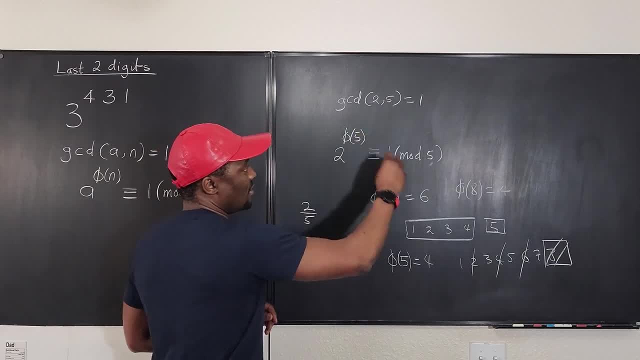 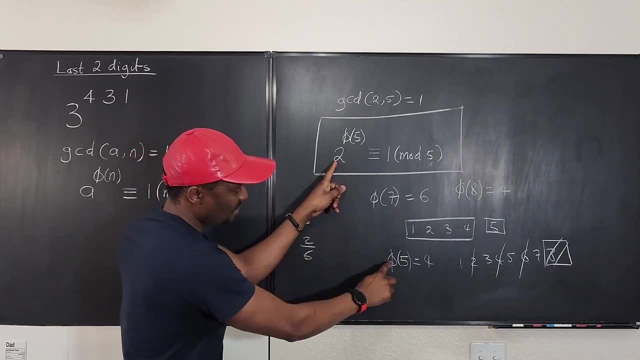 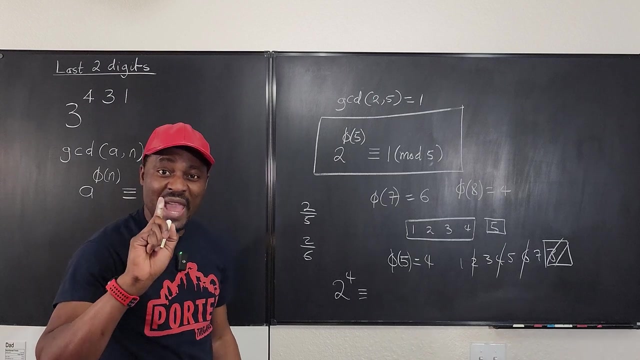 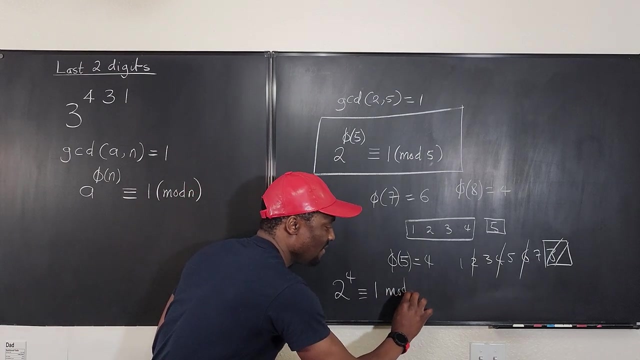 Okay, Which means? so? what does this interpret to? It means: look at this. This means: if I raise two to the phi of five, what did we say? phi of five was four. So if I say two raised to power four, the remainder will always be one if I divide this number by five. That's the meaning of this sentence. This is a mathematical sentence. 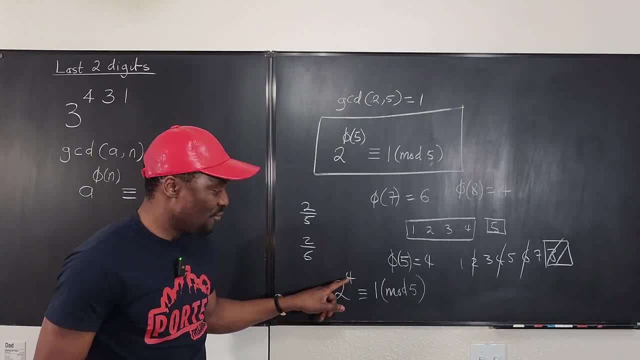 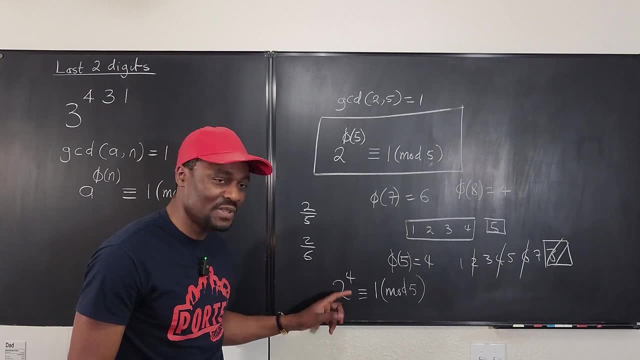 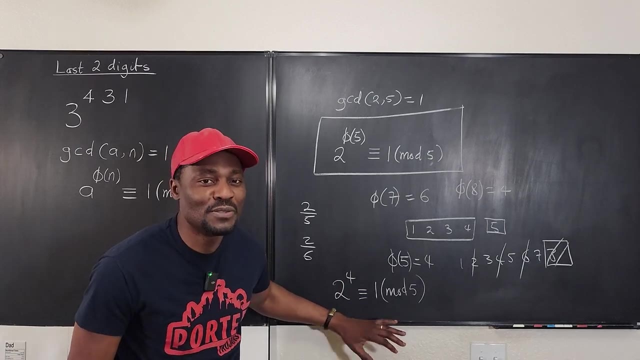 It means when two is raised to power four, the remainder will always be one when you divide it by five. Is this true? Yes, Because two to the fourth is 16.. And 16 divided by five is three remainder one. You will be shocked how useful this is, because that's what we're going to do Now. why do we need to use it? 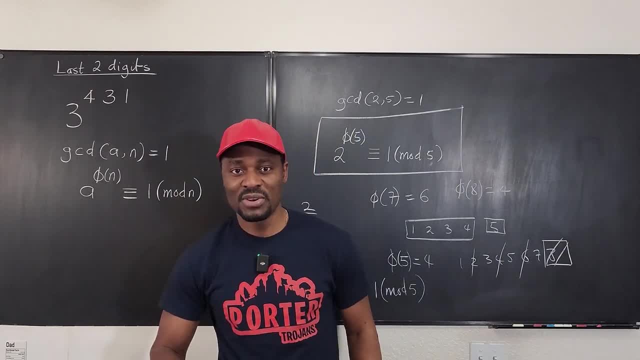 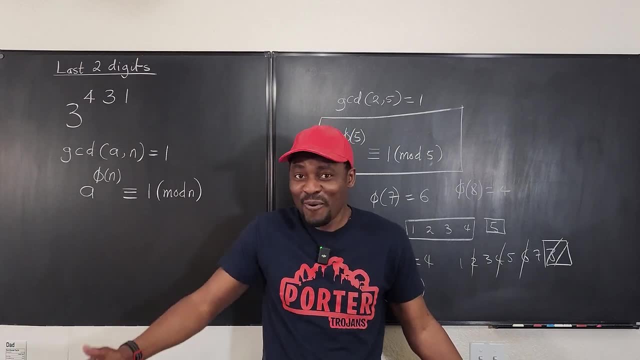 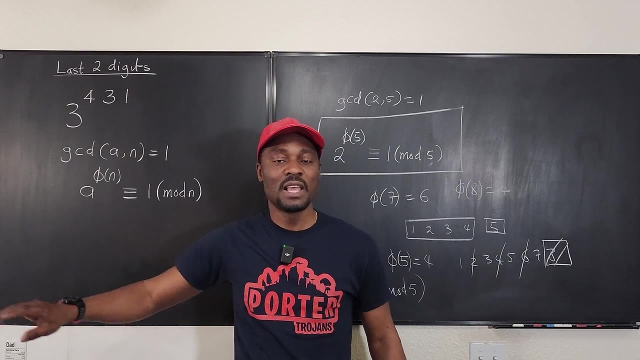 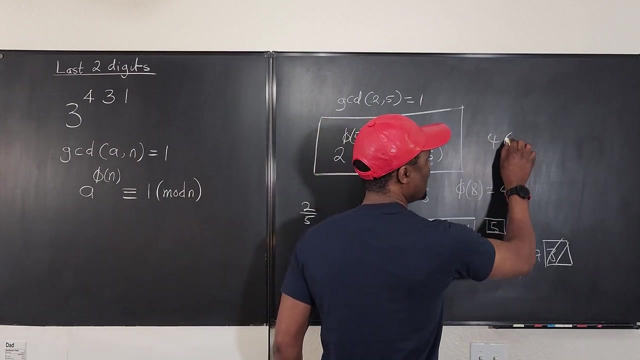 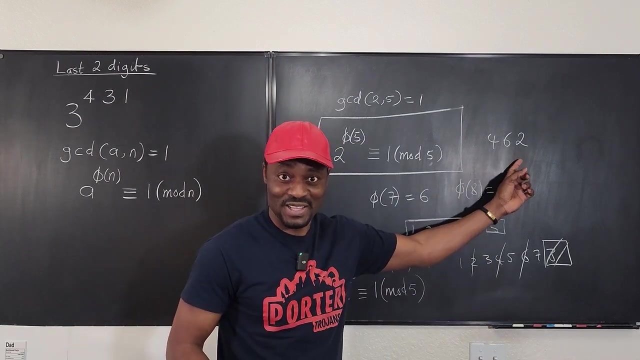 Look, the last two digits of any number is always the remainder when you divide that number by 100.. You see how important this rule is. The last two digits of any number, no matter how big the number is, will be the remainder when you divide that number by 100.. Okay, So if we said four six two, what will be the remainder when this number is divided by 100? The remainder is going to be 62.. Well, which would be the last two digits? six and two. So we can say that four six two will be 62. 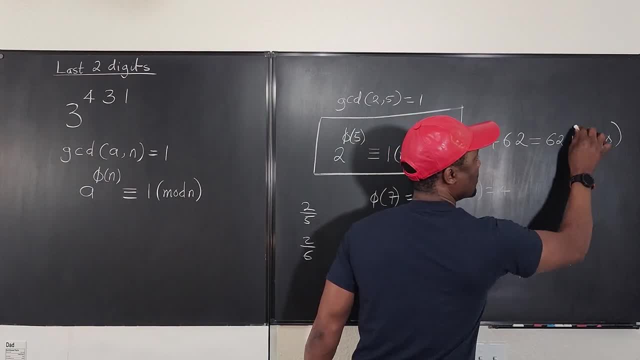 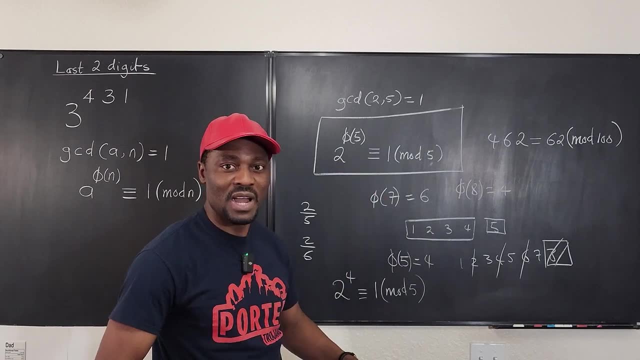 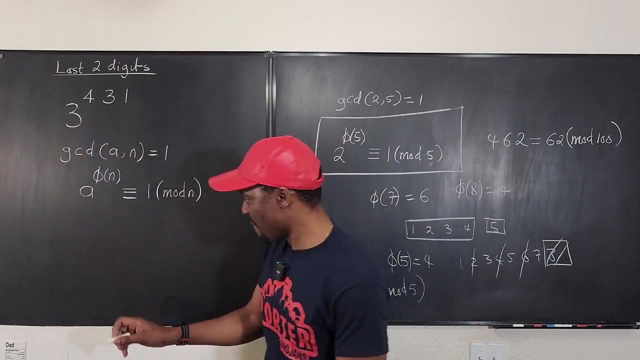 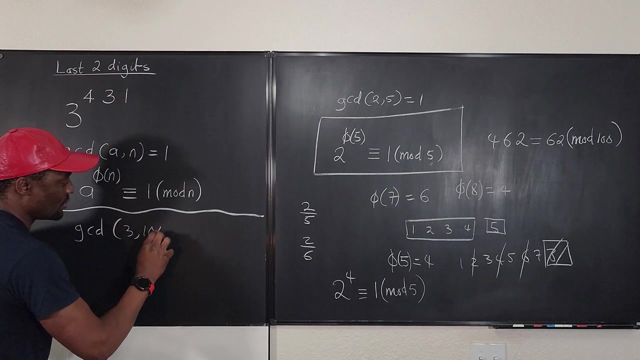 Okay, Now that you see the whole reasoning behind it, let's go use our Euler's Toshin function. Oh, what is the phi of 100?? So now that three look. so if we want to use this, we're going to say that the GCD of three and 100 is equal to one, which means that if we raise three to the phi of 100, we're going to get the GCD of three and 100. 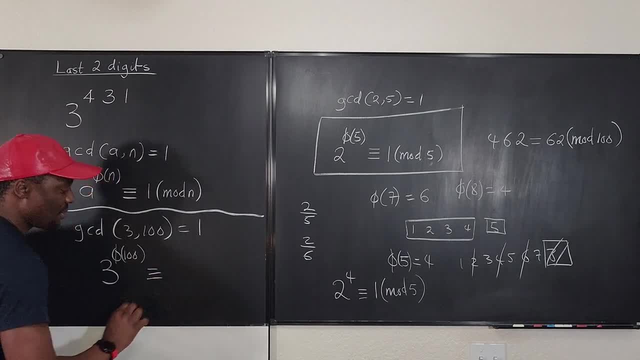 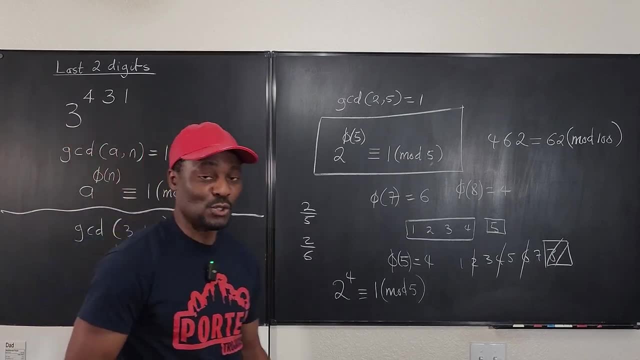 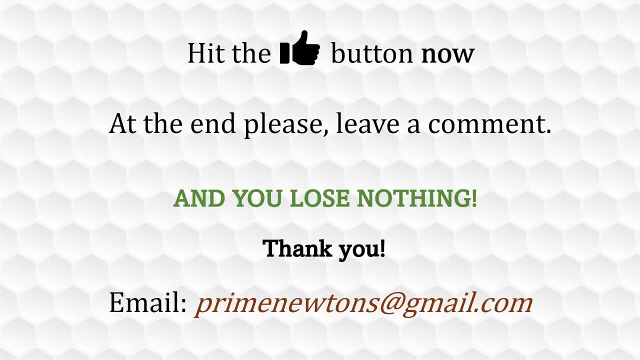 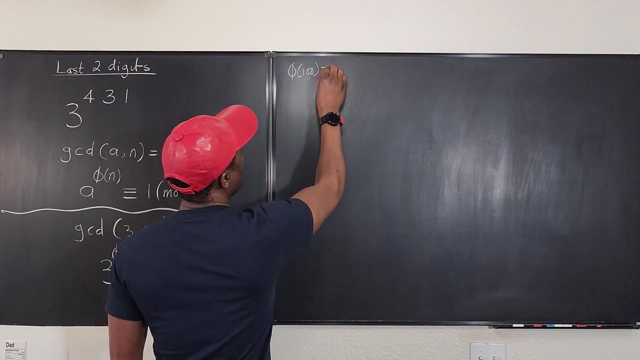 So if we raise three to the phi of 100, it's going to be congruent to one mod 100., And this is a very useful tool for us in finding the last two digits of this gigantic number. Let's do it. The phi of 100 is 40.. Now, in case you're wondering, how did we know it? The formula for this is this: 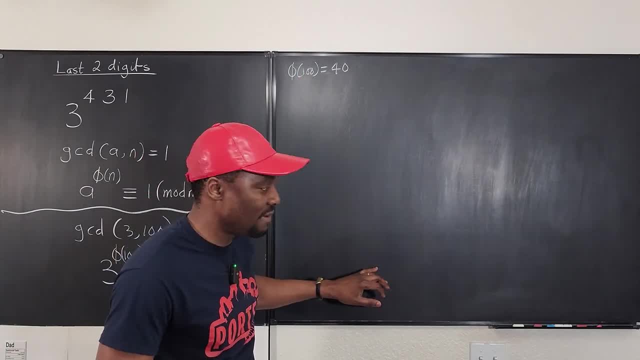 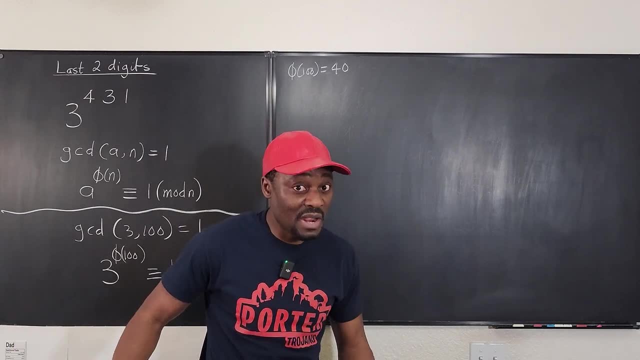 Because this is not a prime number. See the two examples I gave you. I used five, I used seven. Those are prime numbers. So for a prime number, every number before it is relatively prime to it. So you just pick the number less than one. 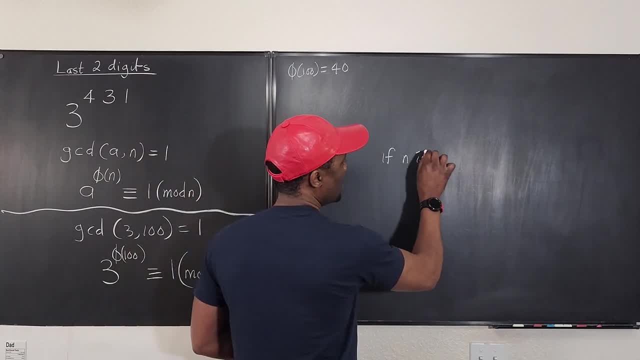 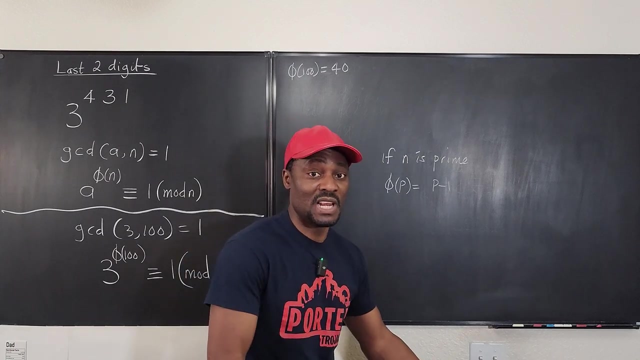 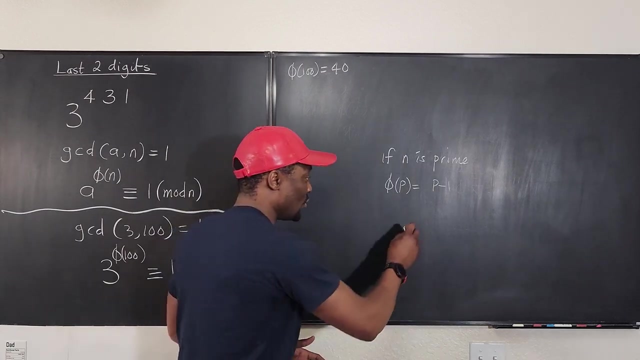 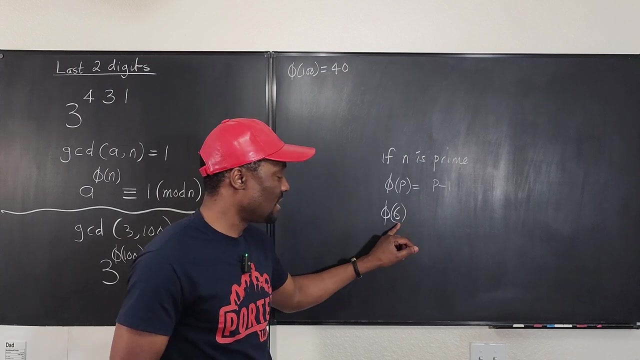 So look at this: If n is a prime number, then the phi of any prime number is equal to p minus one. Just subtract one from that actual number. So the phi of 23 is 22.. The phi of 29 is 28,, because those are prime numbers. Now if the number is not prime, you have to break it into the prime factors. So, for example, the phi of six. you cannot calculate the phi of six using this formula, because this is not a prime number. 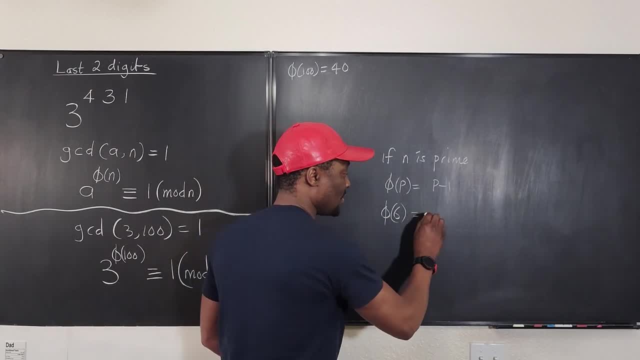 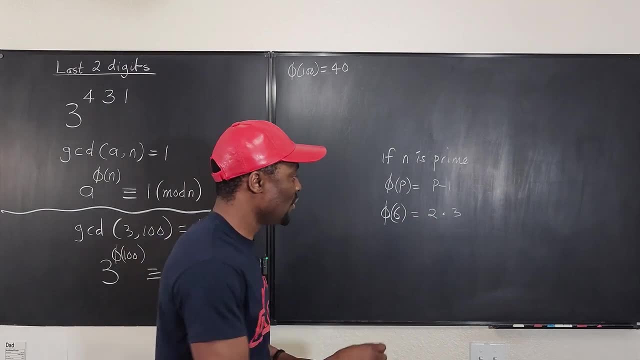 But I can write six as a product of prime numbers, which is going to be two times three. So then I can find the phi of two, find the phi of three and then multiply them together. So it would be the phi of two times the phi. 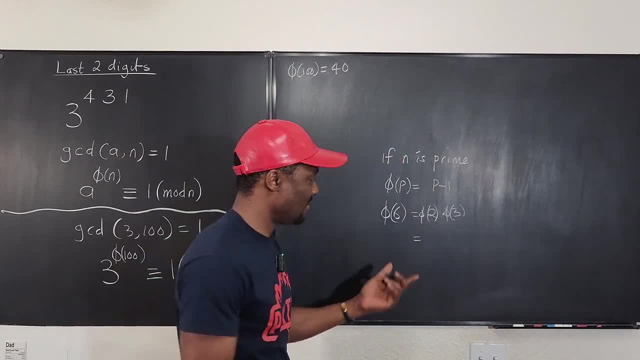 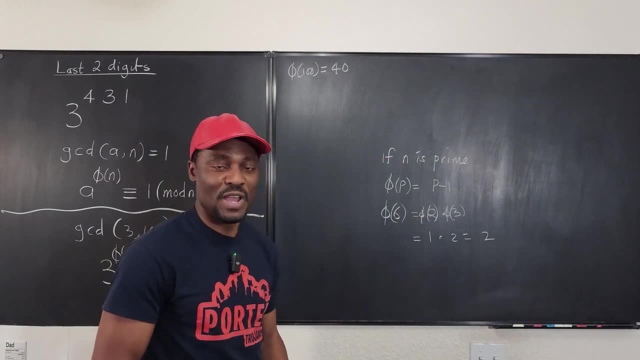 The phi of two. how many numbers less than two? It's one, Here it's two. So the answer to this is two. So the phi of six is two, And you can try it List out all the numbers that are less than six, but they have to be relatively prime. 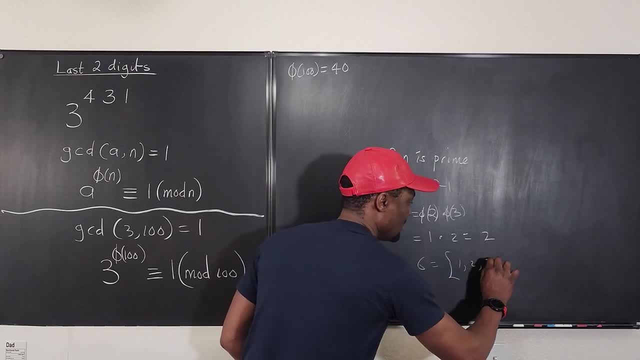 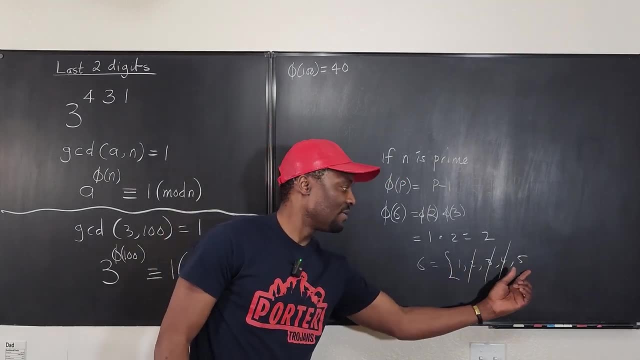 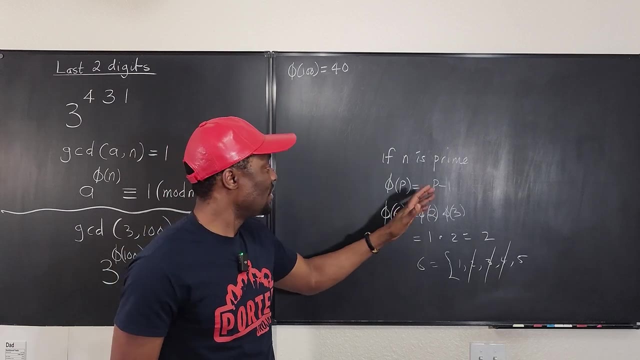 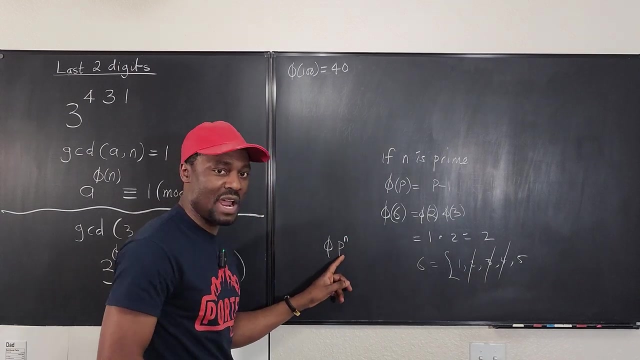 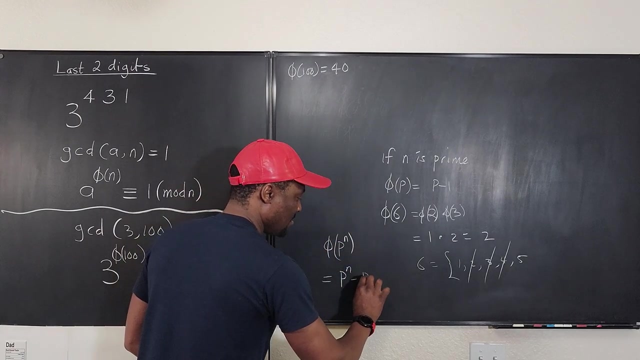 Look, six has a set of one, two, three, four, five. This is not. this is not. this is not because you have to simplify. Only one and five are relatively prime to six. Okay, The formula always works. So the formula for 40, for 100 is the same thing. So now that, however, the phi of p to the n, let's say the prime number, is raised to a power, the phi of this number is basically p to the n minus p to the n minus one. 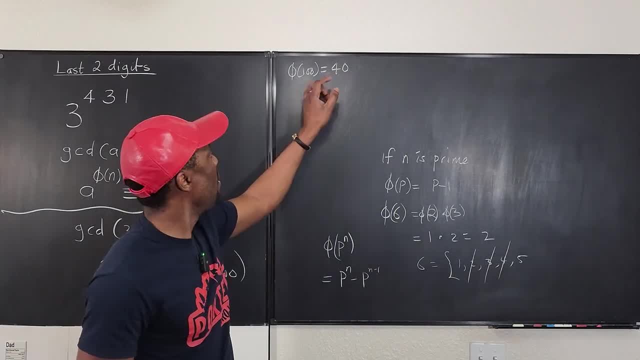 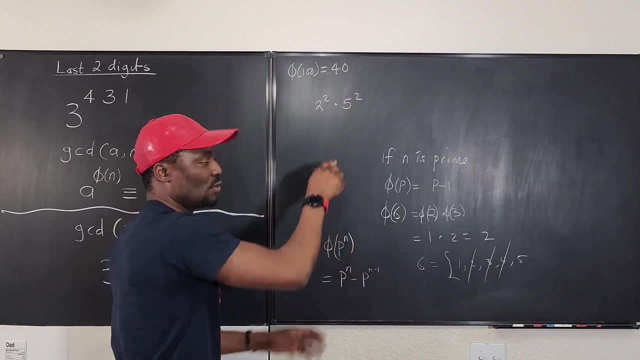 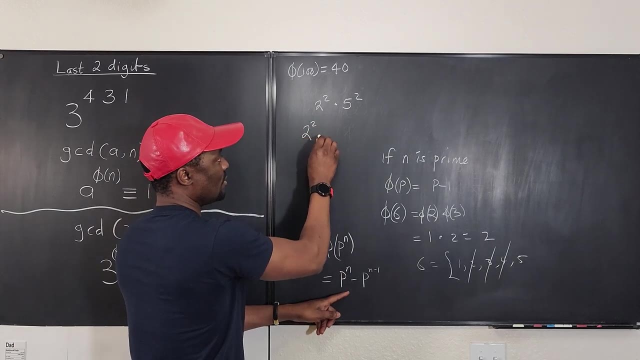 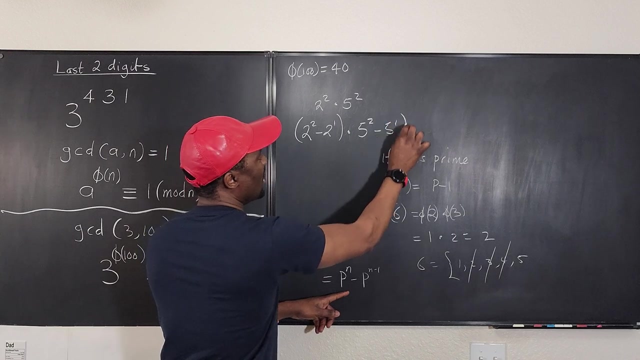 You just reduce the power. So if we do the same thing for 100, it's going to be two squared times five squared, Because two squared times five squared is what gives us 100. If we try to find the phi of this now using this formula, it's going to be two to the two minus two to the one, multiplied by five to the two, minus five to the one. 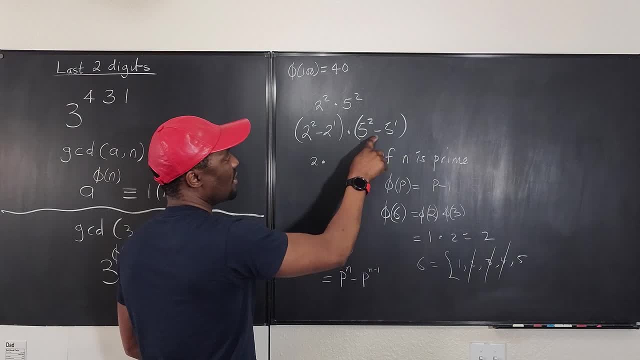 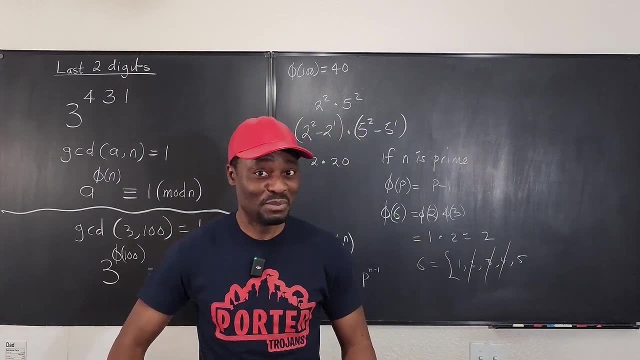 This is going to be four minus two, That's two. There's going to be 25 minus five, That's 20.. So two times 20 gives us 40. And that's the phi. Well, I had to show you because I know some people will be wondering: how did he get 40?? Okay, that's how I got 40 in other videos. 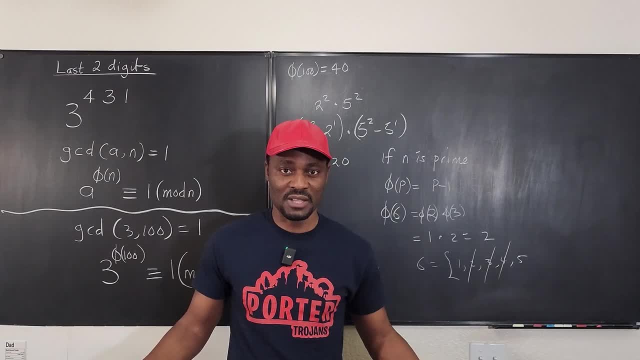 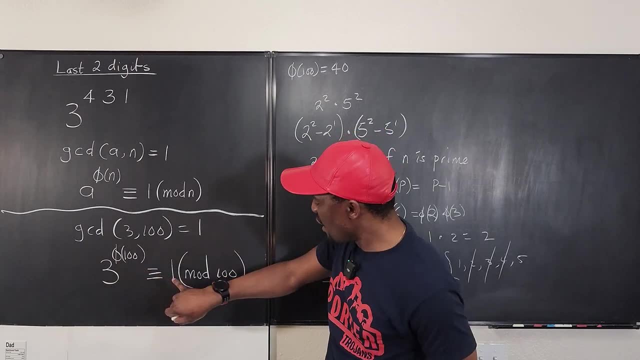 Okay, I'm going to go in depth into number theory and explain some of the concepts, But for now we've gotten the ingredient we want. We know that if we raise three to the 40th power, it will always leave a remainder of one. That's a powerful tool. 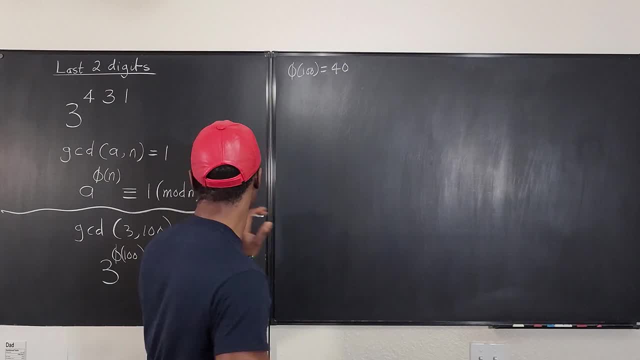 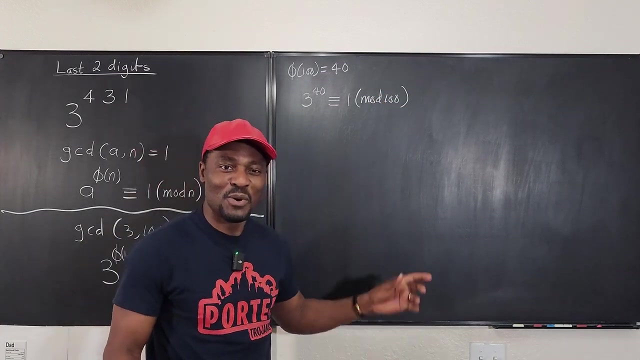 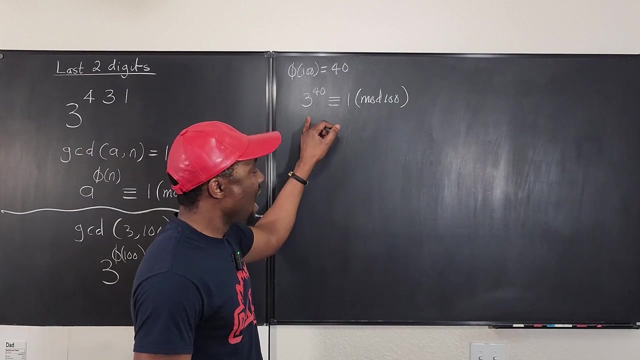 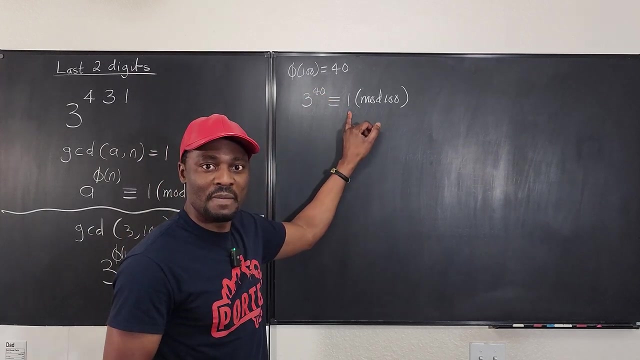 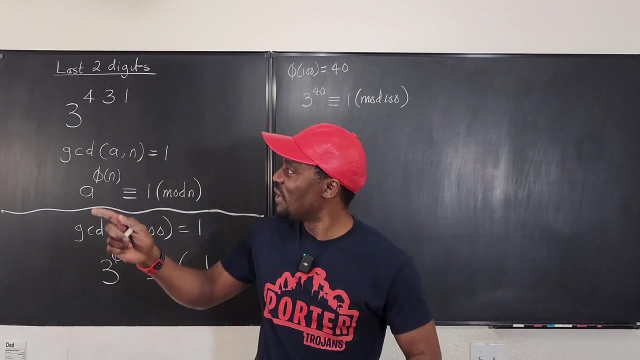 Okay, now that we know the phi of 100 to be 40, we can just go here and say that three to the 40 will always leave a remainder of one when it is divided by 100.. Okay, Do we know three to the 40?? We don't care, But we know that Euler's theorem. Okay, I don't need to know three to the 40.. Now watch this: If I multiply this by another three to the 40, the remainder is still going to be one. I multiply it again: the remainder is still going to be one. So how many three to the 40s do I need to do? if I have to go 431 times, That's it. So what you need to do now is to go 431 times. 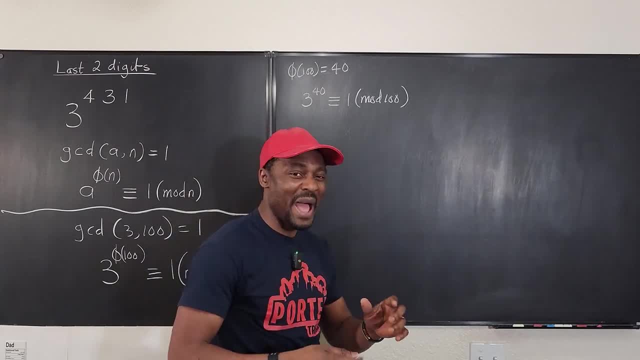 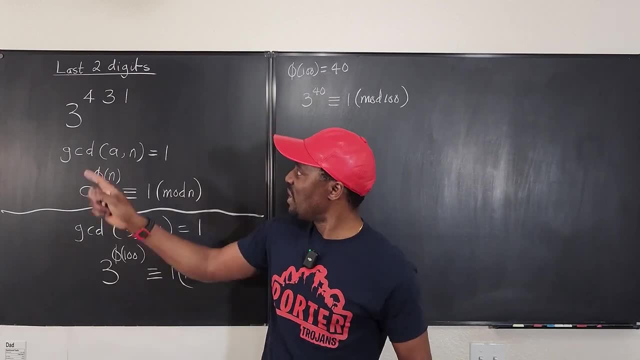 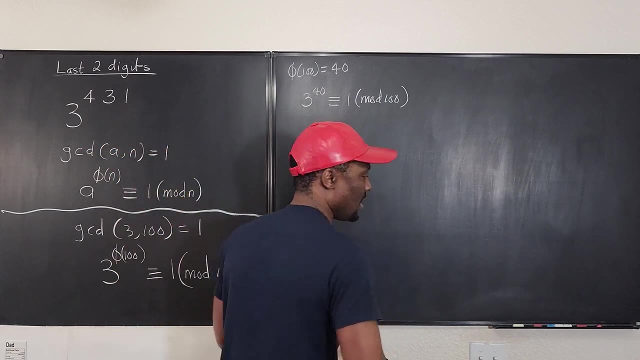 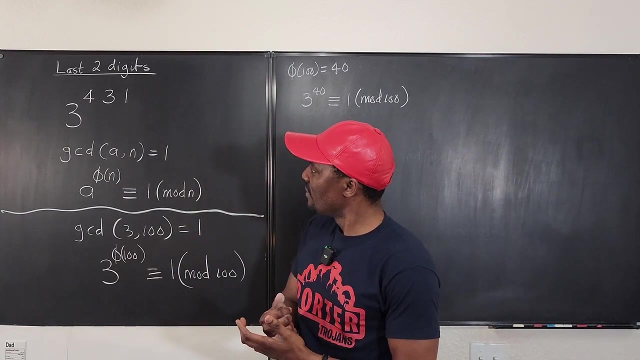 That's it. go back to your. okay, now we have to do algebra. okay, go back to your algebra one, the laws of exponents, and break this down into multiples of 40. okay, so you notice how many times of 40 divide 431. well, 440 would have been a good number, that's 11 times. but i mean, is it 11? yeah, 11 times, but we 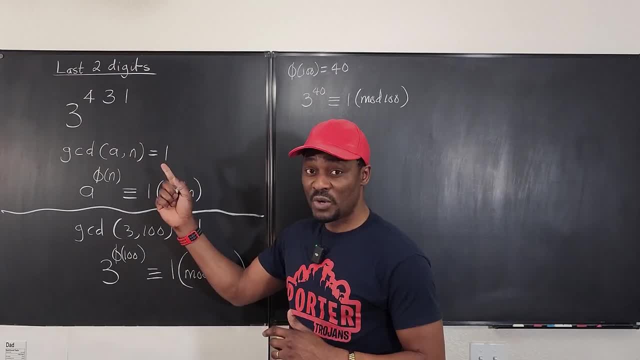 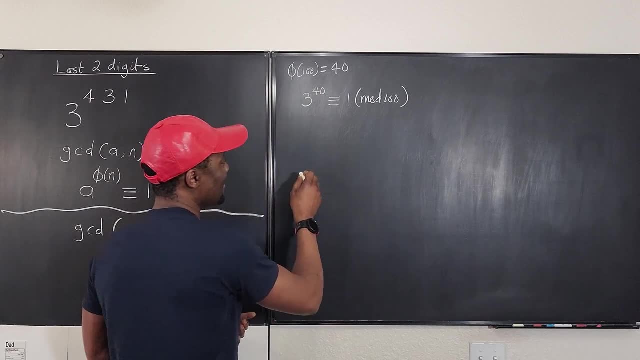 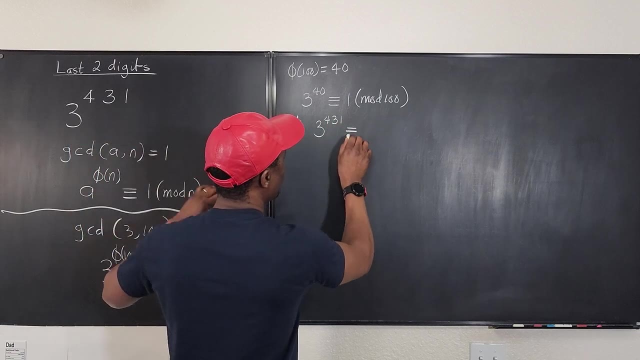 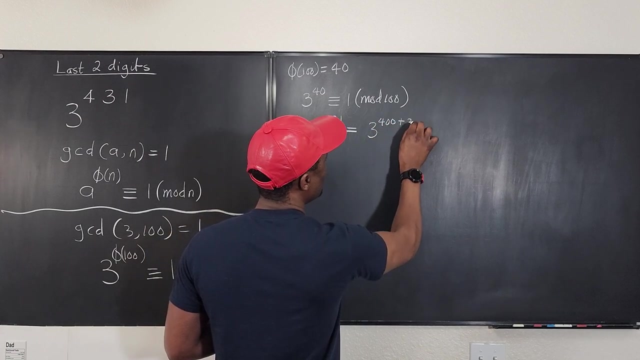 can't get 440, here we can. you have to be less. so we know that 40 will divide 431 10 times right? so we can write this as: let 3 to the 431 be equal to 3 to the 40 or 3 to the 400 plus 31. i think that's a nice way to write it. 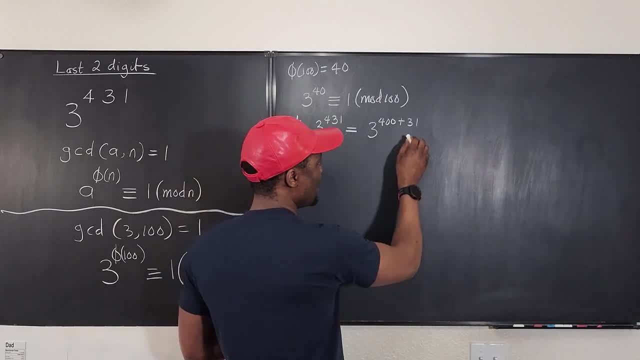 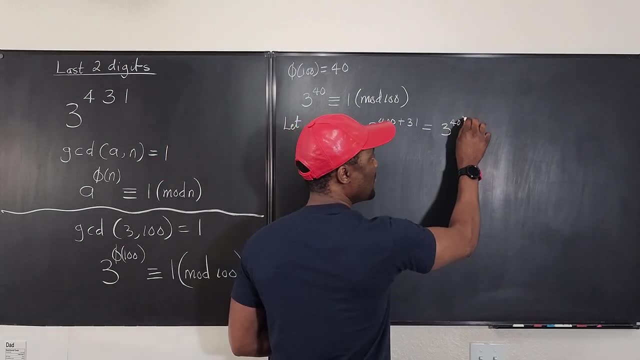 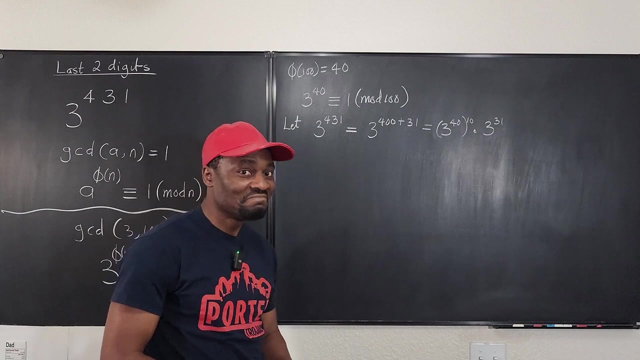 okay, if you do this, then this is going to be equal to 3 to the, since we need to generate multiples of 40. so we're going to say 40 raised to power 10 times 3 raised to power 31. you see now, if we write this, modulo 100. 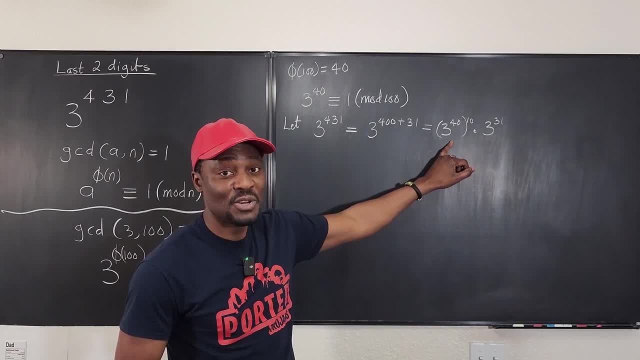 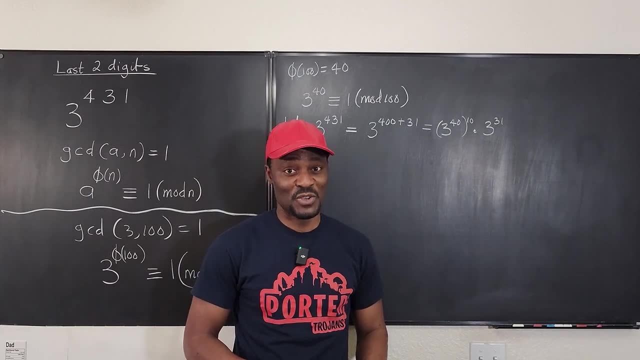 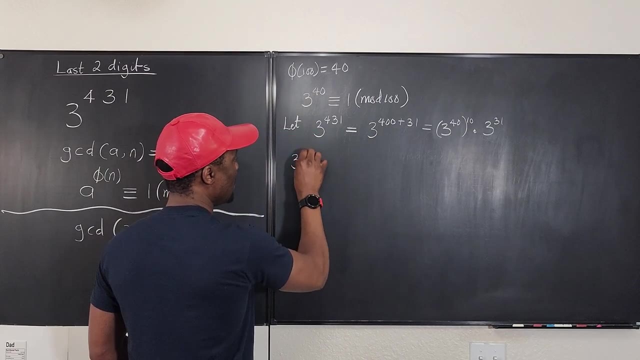 you know what this is going to be. it's going to be 1. we have reduced this giant number to just 3, raised to power 30. so we're going to be equal to 3 to the, since we need to generate multiples of 431, which makes life so beautiful. okay, so now we're going to say 3 to the 40, raised to power 10. 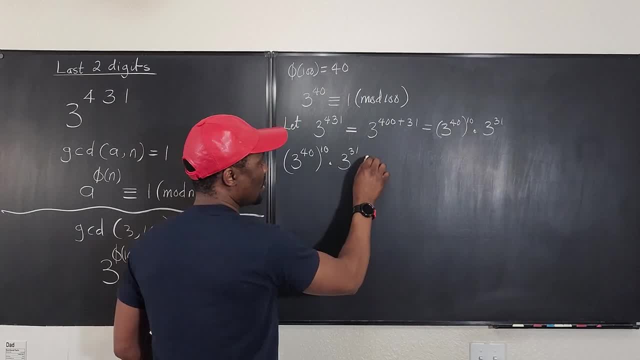 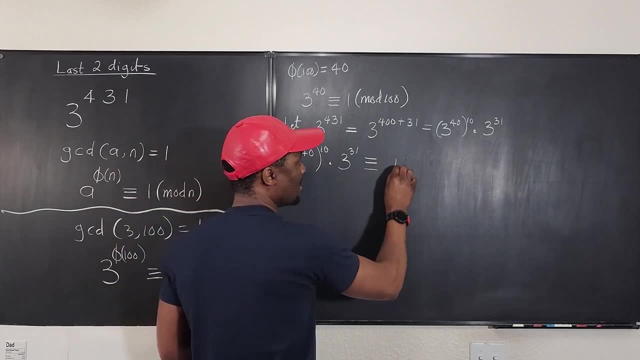 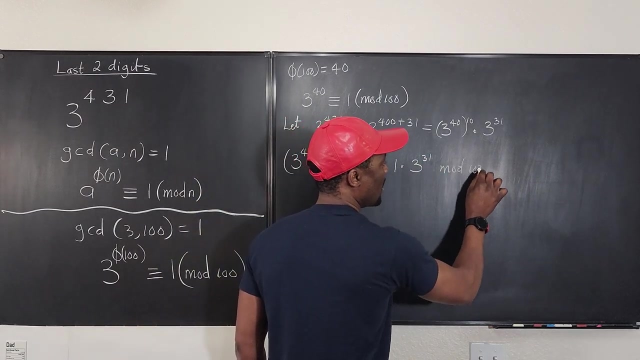 times 3 to the 31 is congruent to this: is congruent to 1 times 3 to the 31, if you're writing it modulo 100. just because of this euler's theorem, we have reduced that giant number to this. now let's say: 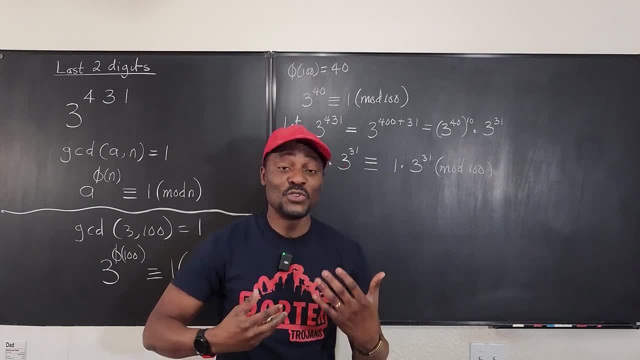 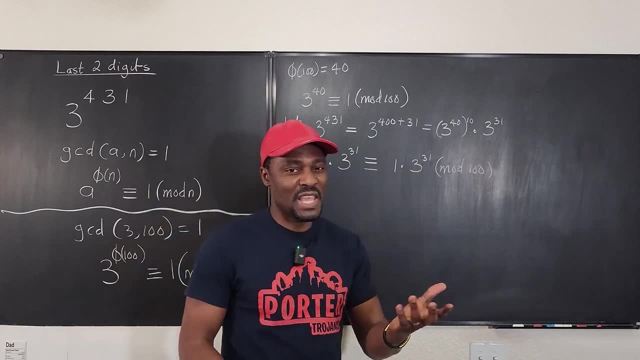 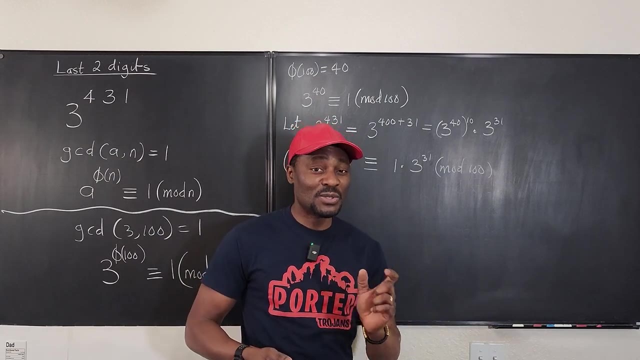 another reduction we can do now. this one- i know you may not know, but i know this one- okay, when you raise 3 to power 4, you get 81. 81 is a big number, but you can use it. okay, but why don't we go higher? when you raise 3 to power 15, guess what the last two digits will be? you can use a. 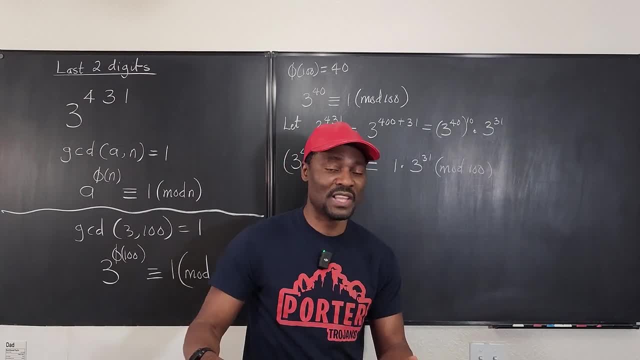 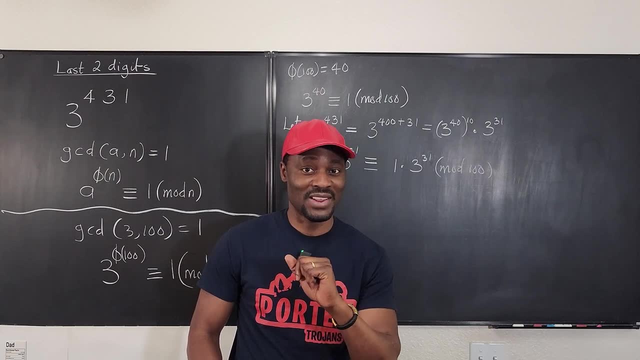 calculator to do that just three times, three times three. keep going until you get to the 15th time. you'll notice that the last two digits it's going to be seven zero seven. that's a skill you want to put in your pocket, or you can just do it manually. it's always it's easy to do, okay, so 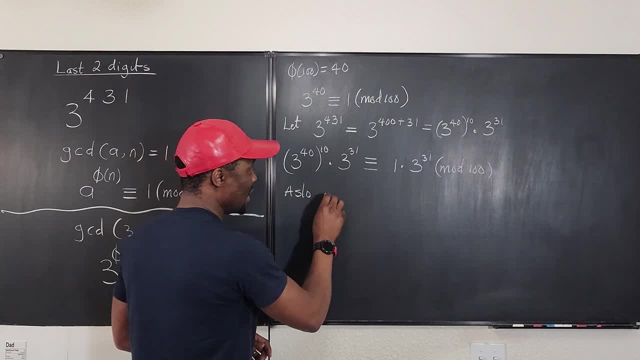 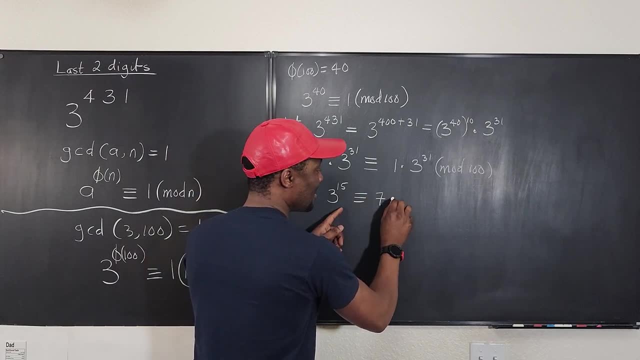 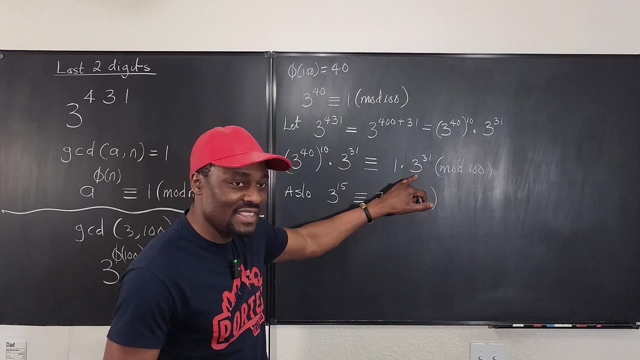 i know also, i know that three raised to power 15 is the same thing as seven modulo 13, modulo 13 modulo 13 Modulo 100. So what I'm gonna do is I'm going to rewrite this as 3 to the 15 twice, and then there's gonna be an extra. 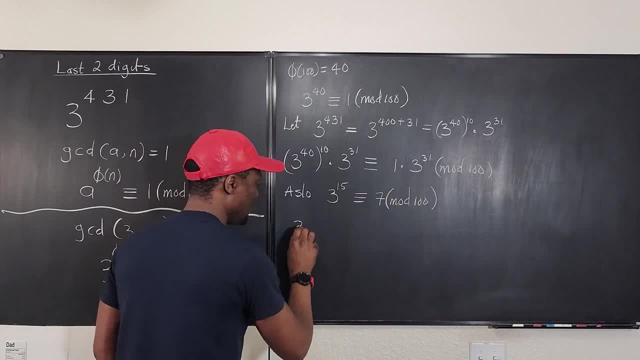 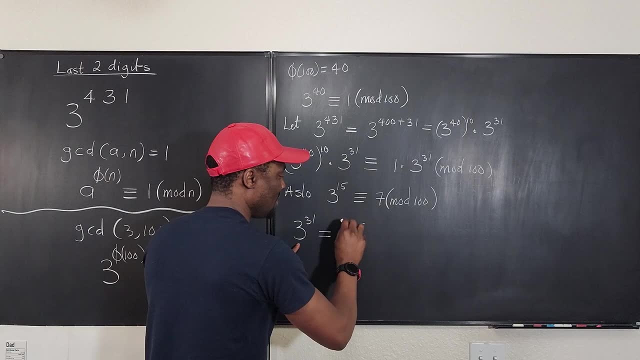 So so I can now say 1 times This is 3 to the 31. But this 3 to the 31 I can write it as 3 to the 15. You see that Race to power 2. or let's write 3 to the 30 plus 1 first, 3 to the 30 plus 1. 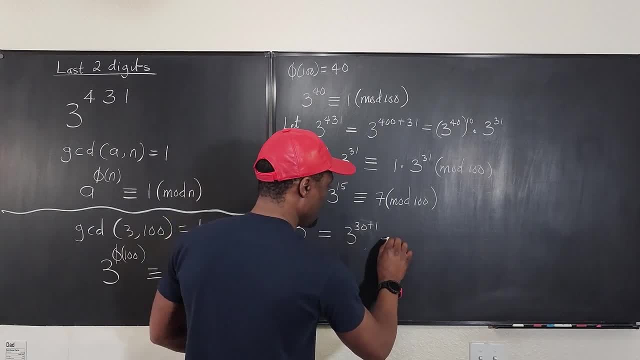 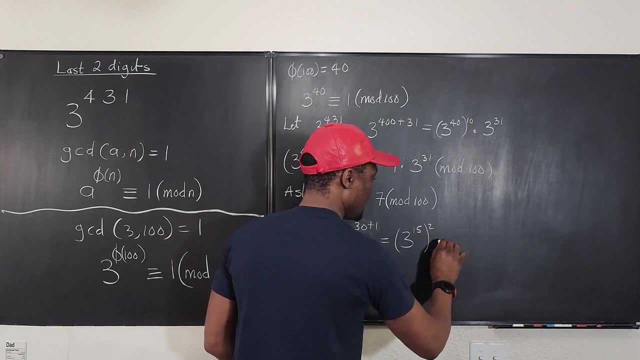 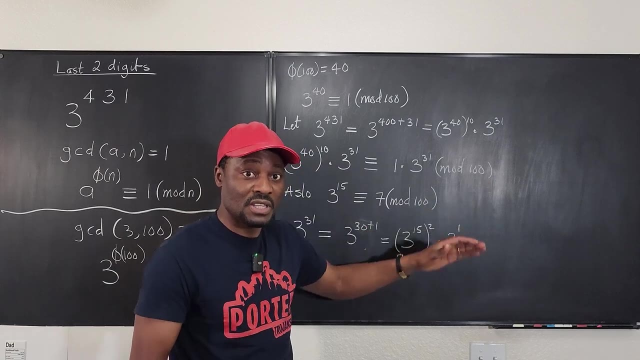 Okay, which is going to be equal to 3 to the 15 Times 2, which is squared, multiplied by 3 to the first. Okay. now I'm going to take this again to modular 100, because I want to find the last two digits.